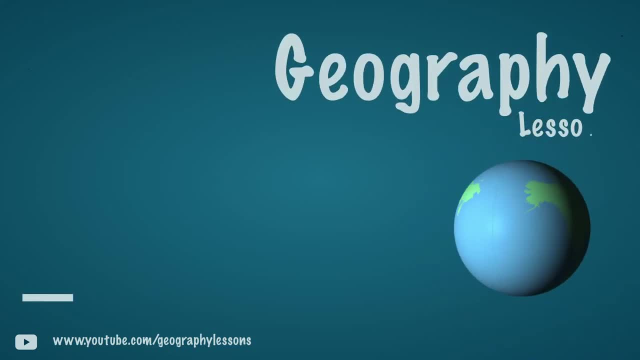 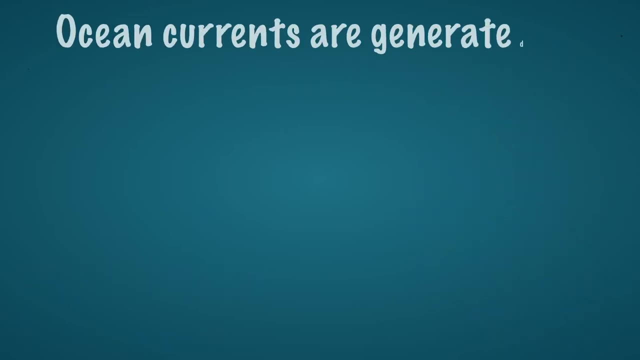 The ocean currents and sea currents are called the oceanic circulation, and they are driven in two ways. The first reason is that the ocean currents on the surface are driven by the wind. The other drive is the thermohaline circulation, which will be discussed first. 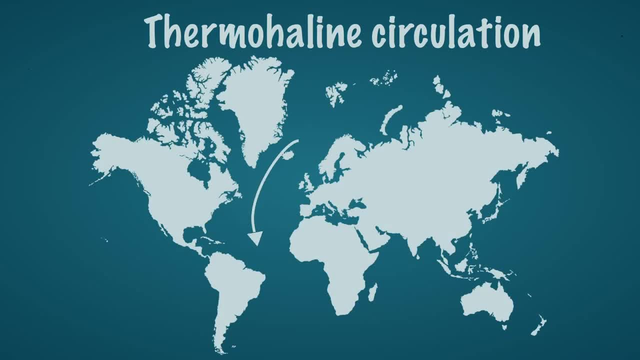 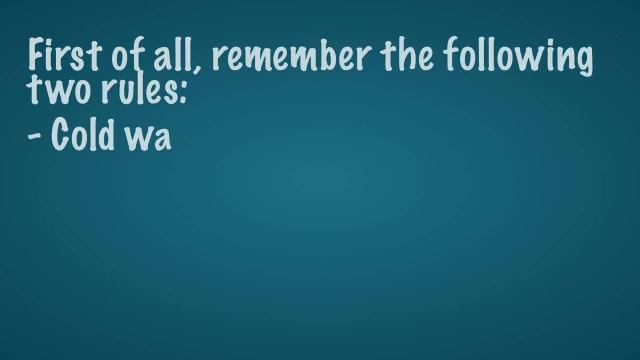 Thermohaline circulation means that the sea currents are driven by density differences of the water caused by temperature differences and differences in salinity. Thermo refers to temperature and haline refers to salinity. First of all, remember the following two rules: Cold water has a higher density than warm water and sinks to the bottom. 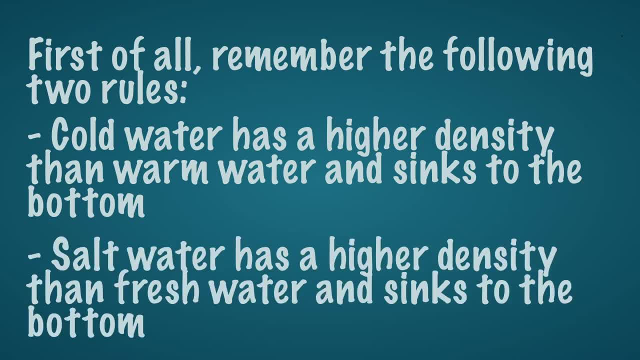 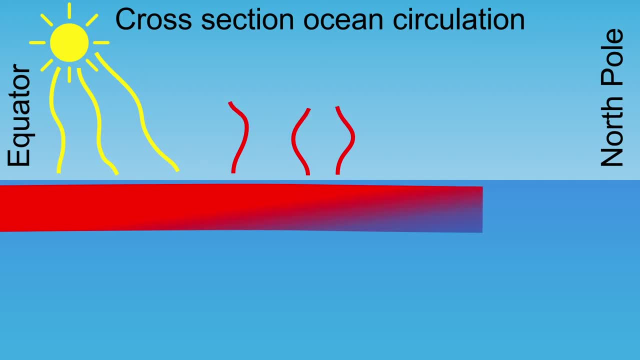 Salt water has a higher density than fresh water and sinks to the bottom Sea. water warms up at the equator, Then it flows towards the North Pole. Along the way, the ocean currents emit a lot of heat, which warms the atmosphere but cools the water itself. 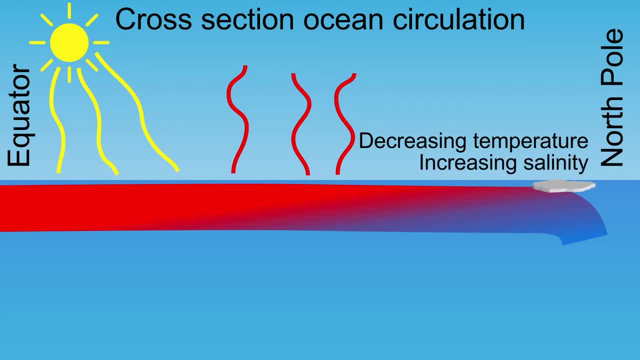 Also, a lot of water evaporates, But the salt remains behind. When sea water freezes and forms sea ice, the salt also remains in the sea water. In short, the density of the water is therefore increasing. Eventually, this water sinks and forms deep water, causing ocean circulation, which is also called the ocean conveyor belt. 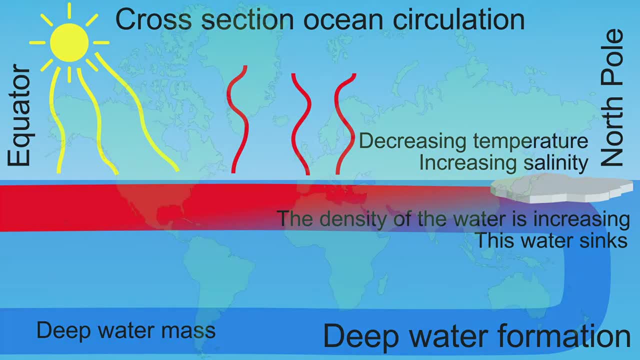 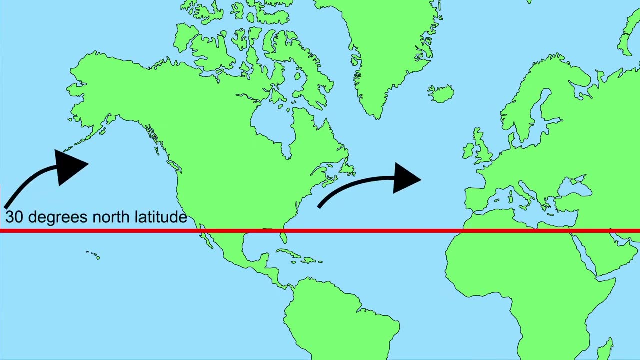 The second driver of ocean currents is the wind. Just north of 30 degrees north latitude there is a westerly wind. The sea water on the surface is blown along But due to the Coriolis effect it deviates to the right seen from the direction of flow. 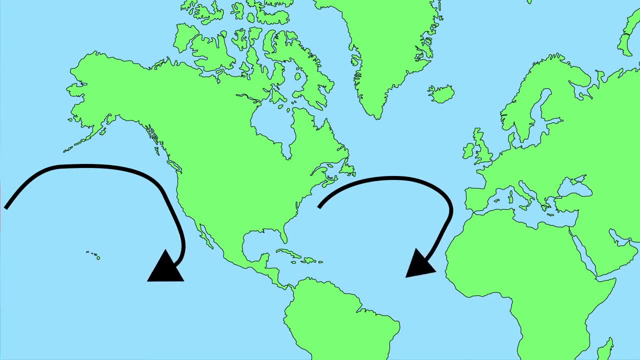 There it is influenced by the easterly trade winds, The wind currents from 30 degrees north latitude to the equator. This creates a circular ocean current, also called a gyre. In this way, two gyres are formed in the northern hemisphere. 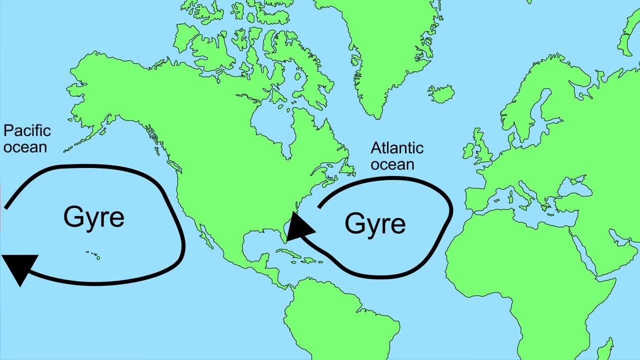 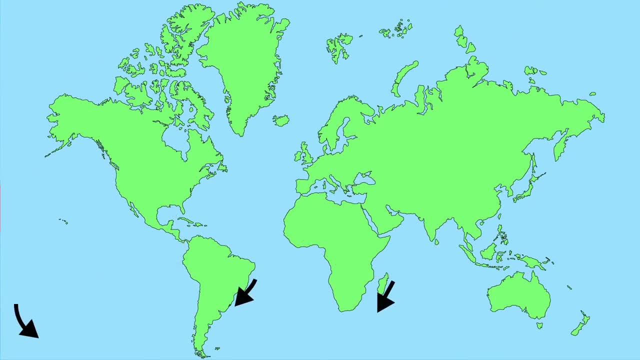 Those in the Atlantic Ocean and those in the Pacific Ocean. These rotate clockwise. In the southern hemisphere the same happens, but in the opposite direction. The west wind, south of 30 degrees south latitude, causes the sea to flow to the east. The sea moves to the left and then follows the trade winds from the east, turning the gyres counter clockwise in the southern hemisphere.